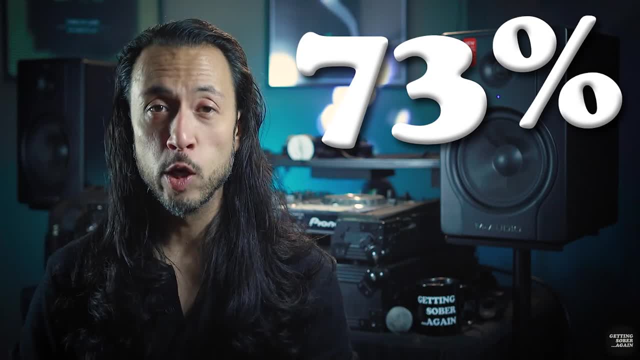 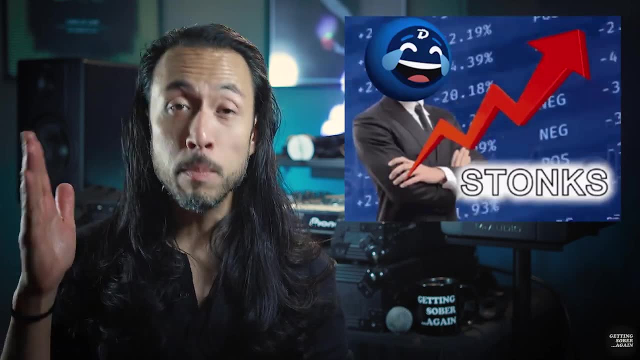 too, thought to themselves that it was too late to start getting sober. 81% of participants said that they've been drinking for 10 or more years Now. whether it's investing your money, your time or investing in yourself, remember that the best day to start anything was yesterday And the next. 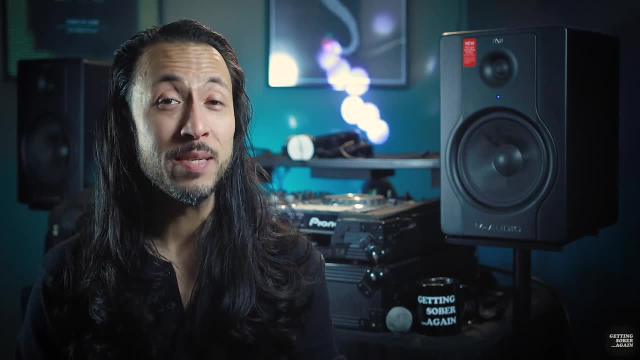 best day to start is today, And if today happens to be the day that you feel inspired to start your sobriety journey, then it's the day to start your sobriety journey. And if today happens to be the day that you feel inspired to start your sobriety journey, then head over to our website. 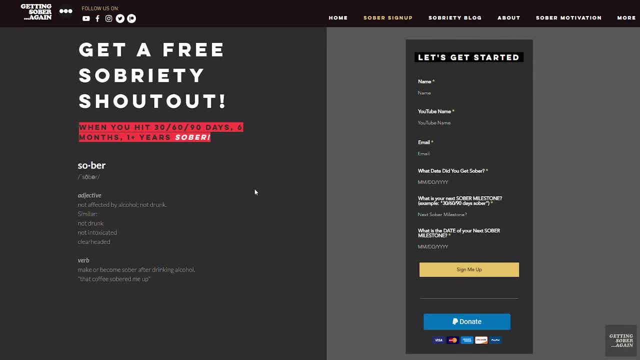 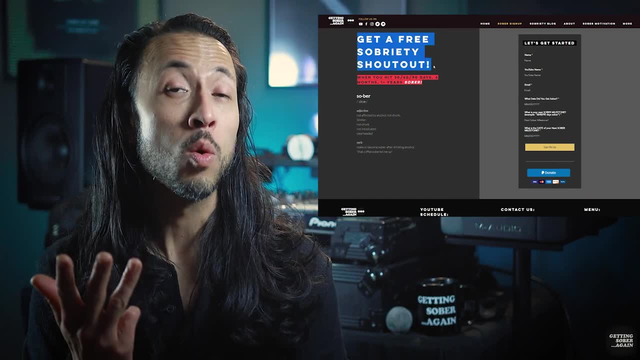 gettingsoberagaincom and tell us what day you got sober, And then we'll shout you out on either your next milestone of 30 days sober, 60 days sober, 90 days sober, six months or one or more years sober Has feeling like a failure kept you from the success that you're looking for. 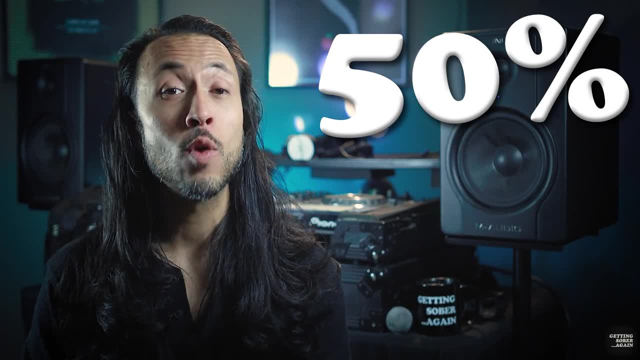 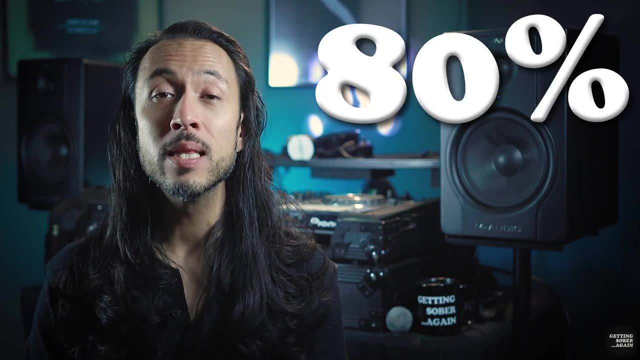 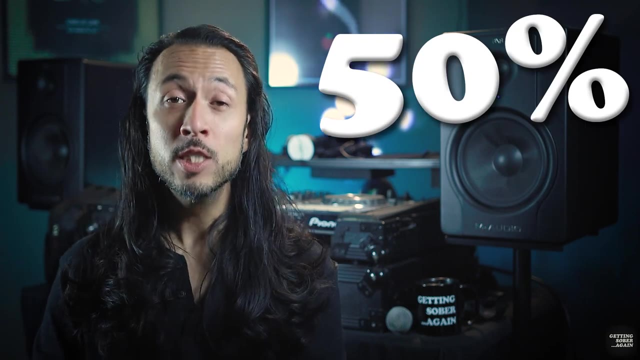 Well, it took 50% of our viewers eight or more times of trying to get sober before actually making the commitment to finally quit drinking. And, with that in mind, 80% of people said that they tried 10 or more times just to try to get sober for one day. Now what about holidays and 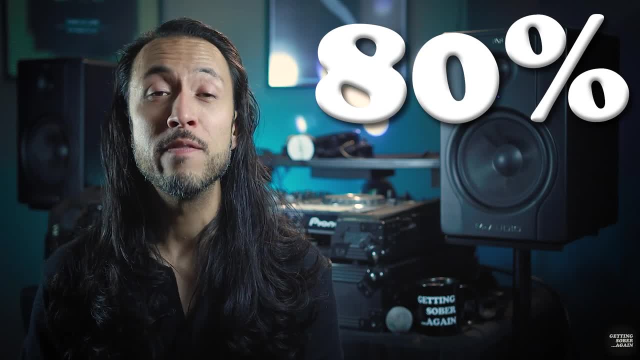 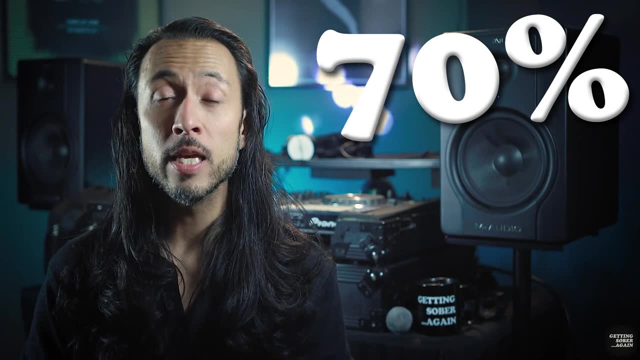 our family. 80% of people said that they typically had five or more drinks on holidays. 70% of people said that they felt guilty about missing quality time during the holidays because they were too hung over to participate. Nearly 20% of viewers said that they still haven't told their families. 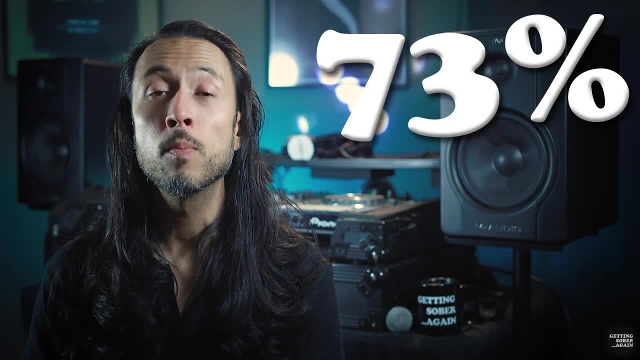 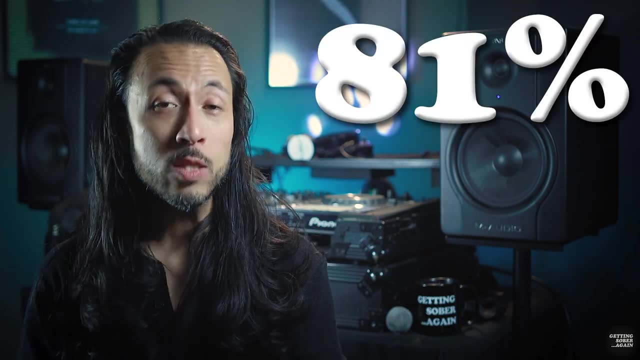 that they decided to get sober, And 73% of people said that they still haven't told their families that they're expecting to be around alcoholic relatives during the holidays. 81% of you said that there was at least one person in your life that would benefit from sobriety, And 62% of you 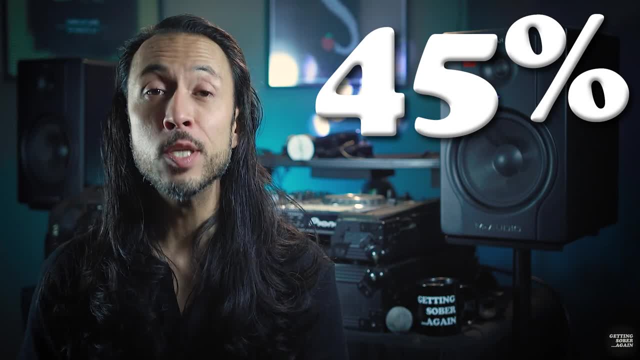 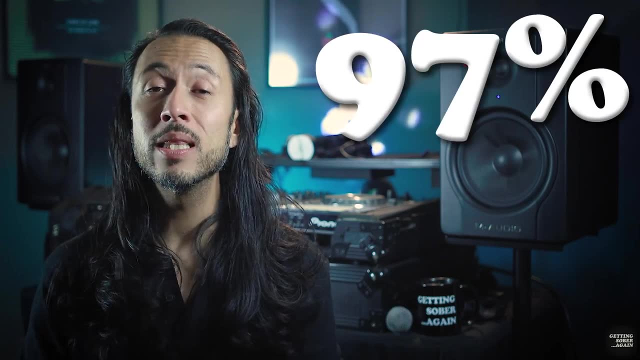 said that it was a family member. 45% of people don't personally know anyone who's sober. So where's the support for sobriety? 97% of our viewers said that they are not currently going to AA meetings and more than 90% of our viewers said that they were not in therapy.